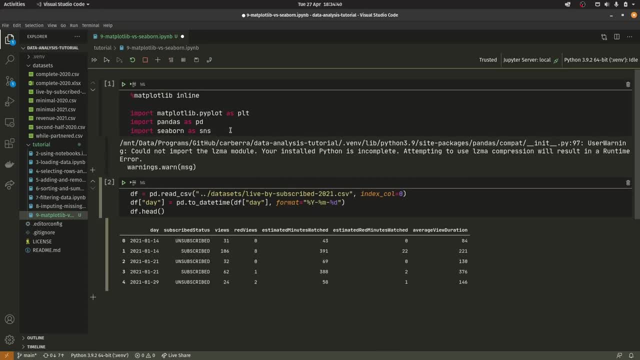 And what I want to show is the differences between Matplotlib and Seaborn. So Matplotlib is Python's graphing library in a sense. At the very least it's its main graphing library. I'm sure there are others out there. 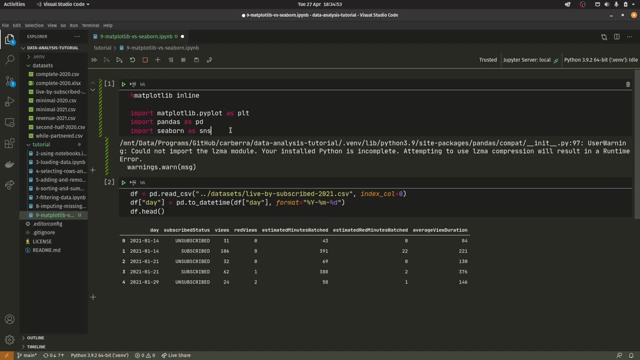 But Matplotlib is the one that really most people use and it is very powerful. You can do a lot with it, but it is also very, very complicated and very, very tricky to use. There's a lot of weird stuff with it that doesn't make a huge amount of sense. 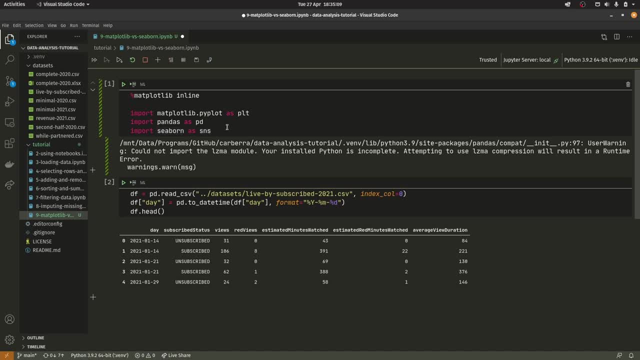 This is where Seaborn comes in. Seaborn aims to be a wrapper that sits on top of a graph. Seaborn aims to be a wrapper that sits on top of a graph. Seaborn aims to be a wrapper that sits on top of a graph. 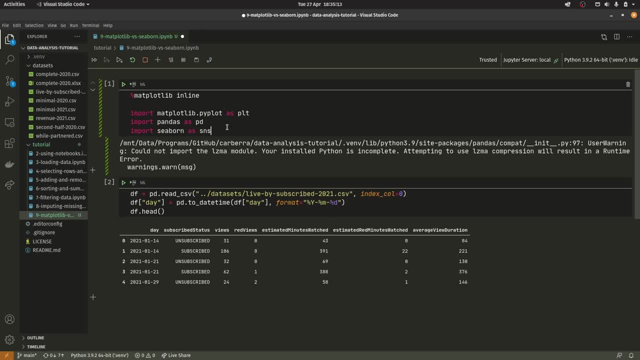 So you're still using Matplotlib, but it just makes everything a lot easier and a lot quicker. Now, if you want complete control, I would probably recommend sticking with Matplotlib. I think you can change Matplotlib settings with Seaborn, but I don't know. 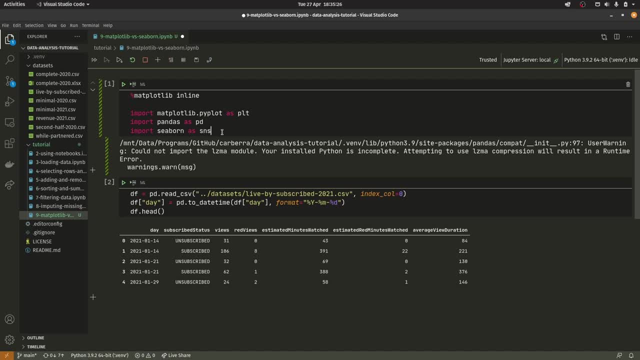 But if you're like me and you just want to get graphs out quickly, you want to see the data there and then then Seaborn is the one to use, And I'm going to be showing you how to make a boxplot specifically. 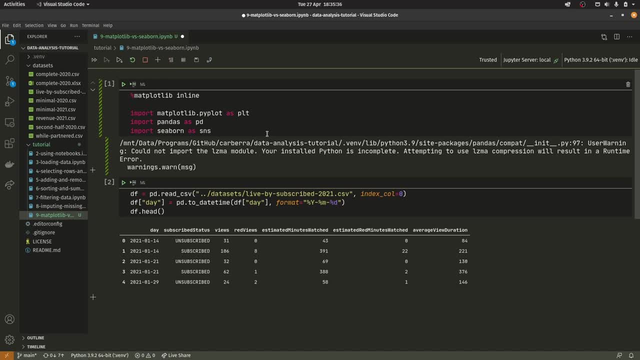 We will get into boxplots in more detail later in episode. What episode is that? It's number 12.. It's a few episodes from now, But for now I just want to show you the differences between how to make a boxplot in Matplotlib and Seaborn. 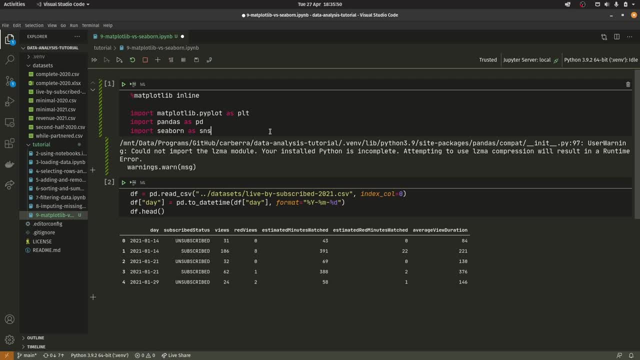 And also differences in visuals, because Seaborn does a lot of stuff with the look as well. So we're going to start with Matplotlib, We're going to come down here and create a cell And we're going to create our figure. 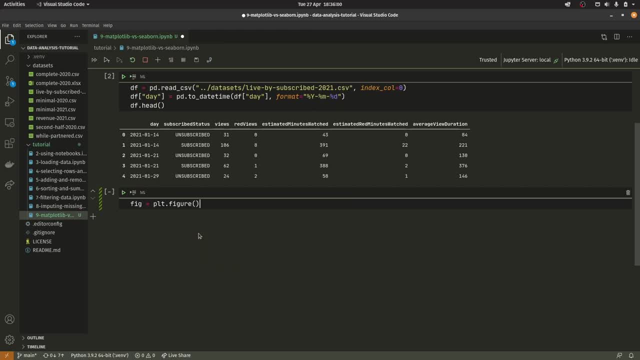 So fig equals pltfigure. Now, regardless of whether or not you use Matplotlib or Seaborn, I'm going to be doing this. You don't have to do it with Seaborn. I don't think. I just like to put everything in a figure, so it's easier. 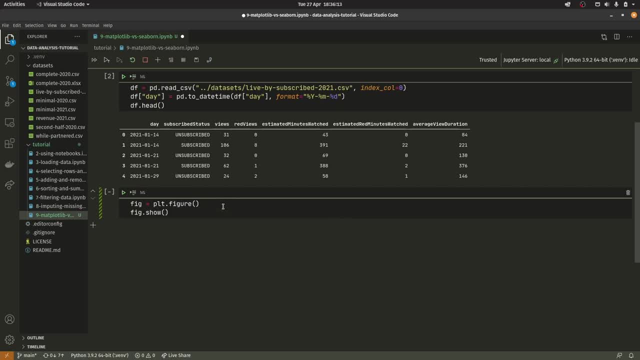 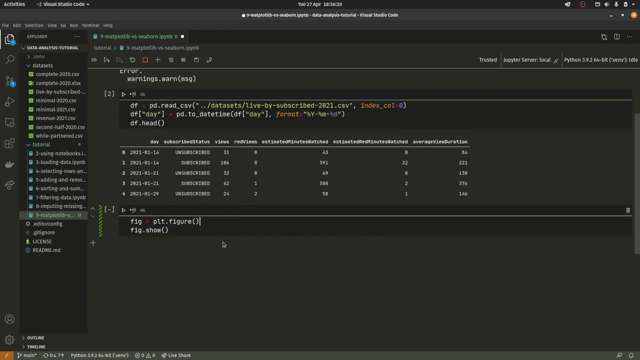 So we can actually do figureshow down here And then everything we do in between that will be adding to the figure And then we can show it at the end And it will show it in the actual thing because we have Matplotlib inline at the top. 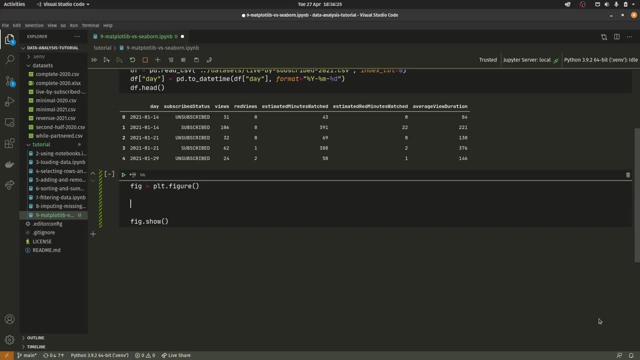 So to create a boxplot- I'm just going to separate it out a little bit- What we do is pltboxplot, And then we open brackets And I'm going to bring down onto a new line and create a list here. So inside this list is all of the different. 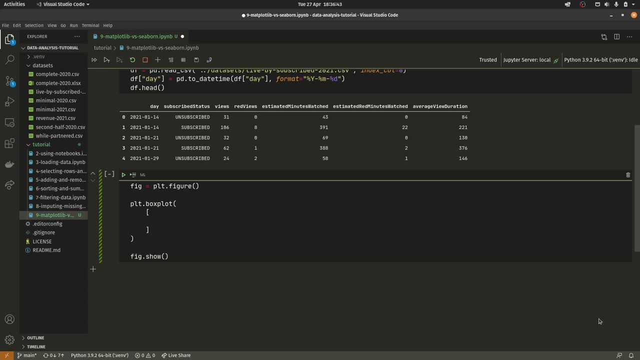 boxes we want to draw. So in this case we want to draw two, And it is dfviews. And then open square brackets again: dfsubscribedstatusdouble equals. Oops, the double equals is there, Subscribed? And then the same thing again. 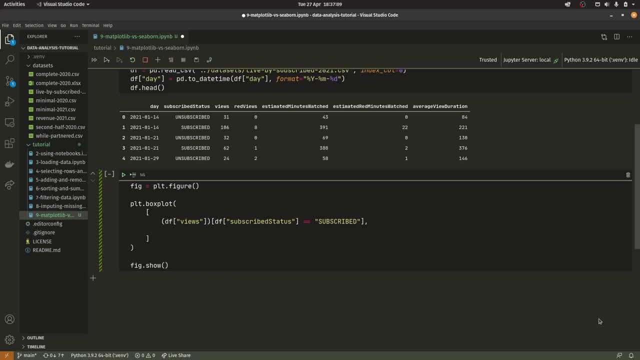 I don't have a left control key at the moment, so I'm probably going to be a bit slower than normal. And then that's a closed bracket there. Do that And then unsubscribe. So what we want to do is we basically want to show a boxplot for subscribed figures and a boxplot for unsubscribed figures. 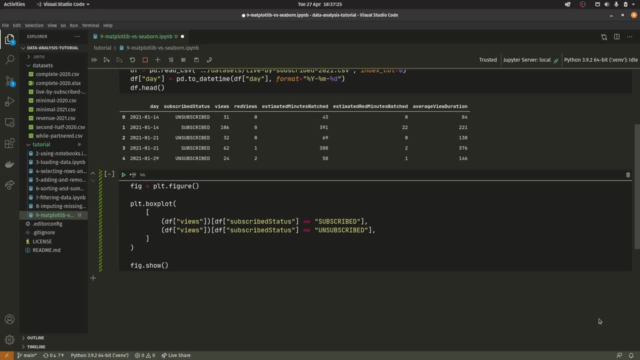 And this is just going to show the views for each in the live streams that I did in January. I can't remember if February is included in that. It may well have been, I don't know. Actually, March may have been as well. 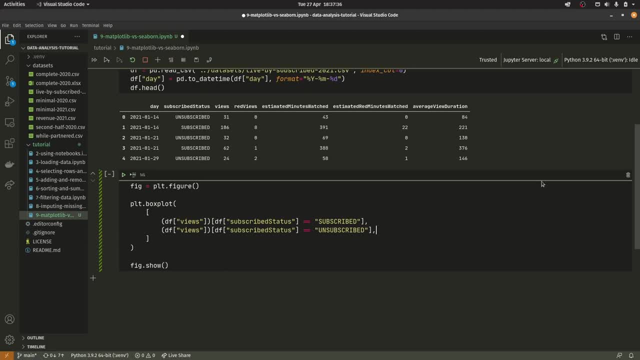 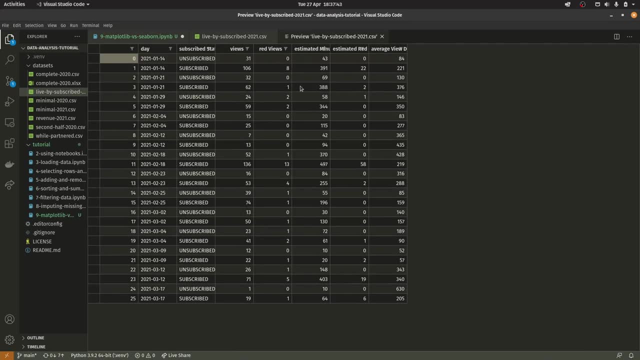 I actually don't remember what's included. We can have a look, actually, Just real quick, All right. So yeah, it's March as well, So you can see, if I open it like this, we have a certain number of views for unsubscribed and unsubscribed people. 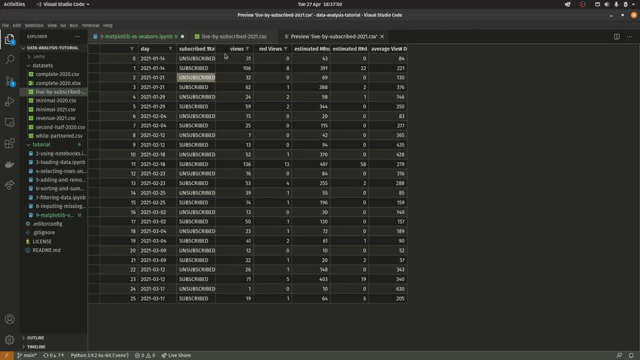 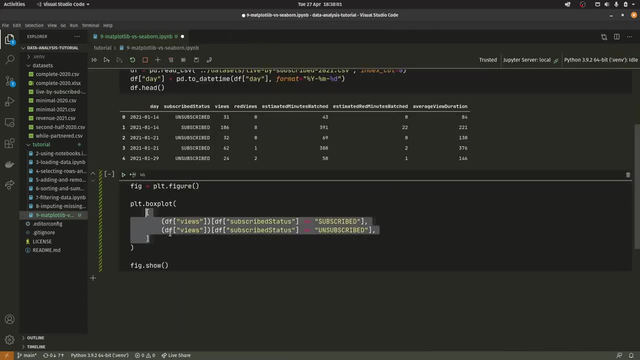 I basically want to show the difference between the two as a boxplot. We want to see how different they are. This is a good way to do that. So, anyway, back to our boxplot. We have the two graphs in there now. 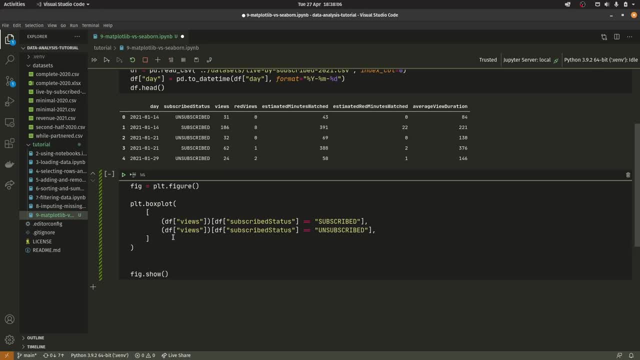 And that's all we need out of that. So now we need to set the x label. So it would be pltxlabel, Subscribe status, if I could spell, which I never can, So I don't know why I keep mentioning it. 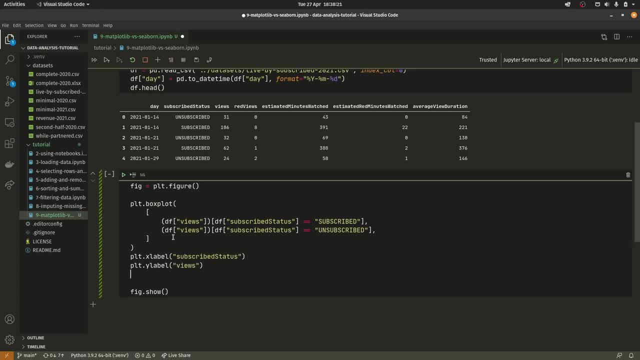 Then we want to set our y label, So the one on the y-axis is going to be the number of views. Then we want to set the ticks. So this is, I believe, the ticks. Yeah, this is the ticks going on the x-axis. 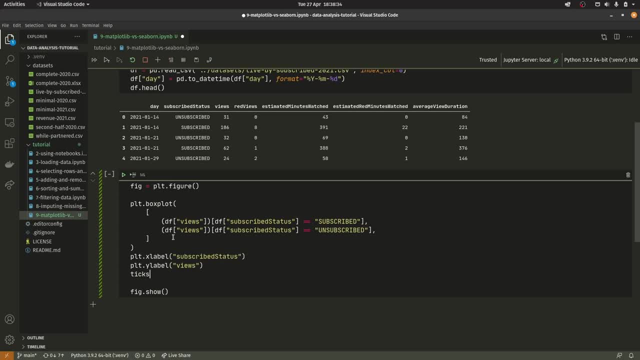 So we want to set kind of what it will read for each thing. It'll make more sense when you actually see it. So we want to set that to a set of df Subscribe status. So we want the- you know subscribed and unsubscribed. 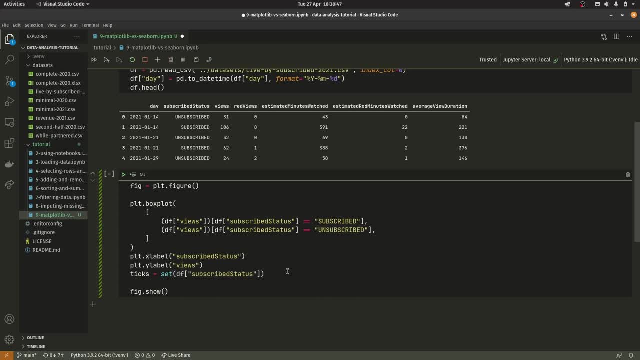 We can have it as a list in there if you want. but I'm just using a set because it makes it just a little bit more dynamic And then we actually need to apply that. So pltxticks Ticks equals range one, len ticks plus one. 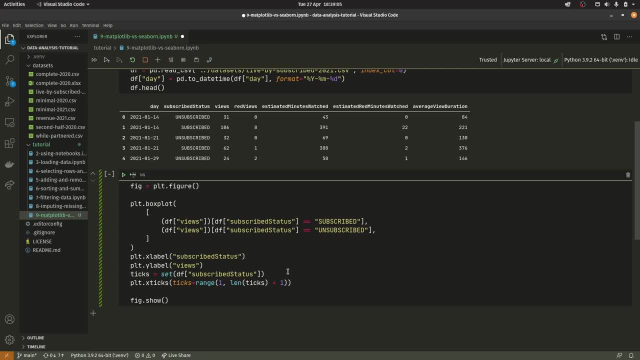 So these are the ticks that we actually want to override, And then we want to set the labels of those ticks to ticks, And that's it actually. So now, if we do control, enter and show it, we can see that this is our graph here. 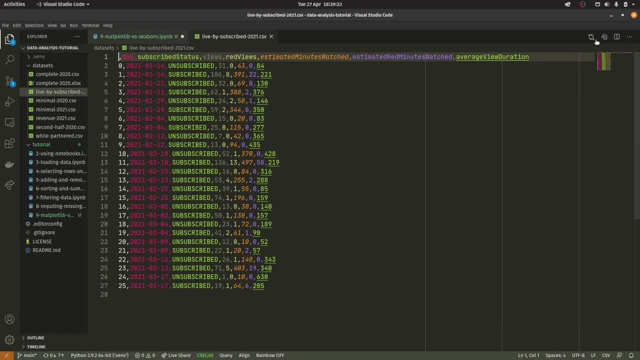 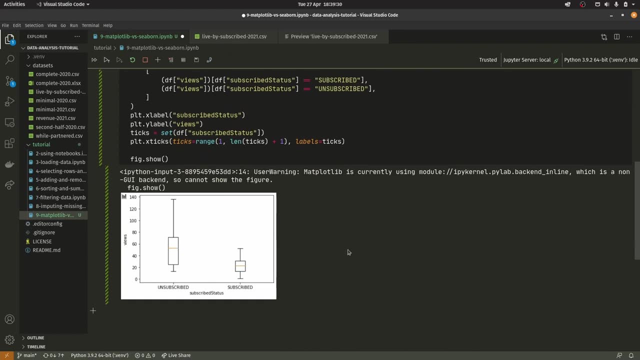 Is this actually backwards? Because I genuinely don't know if this is backwards or not, Because you don't really get a choice: Subscribed is the highest one. It is backwards, Okay. so in this case, we would need to do this. 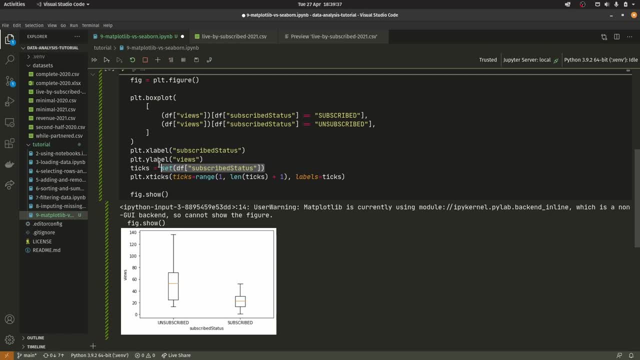 Because last time I did this it wasn't backwards, I guess, because we're using a set, So we actually want this to be subscribed and then unsubscribed. There we go. You can set it as a tuple as well. I'm pretty sure, anyway. 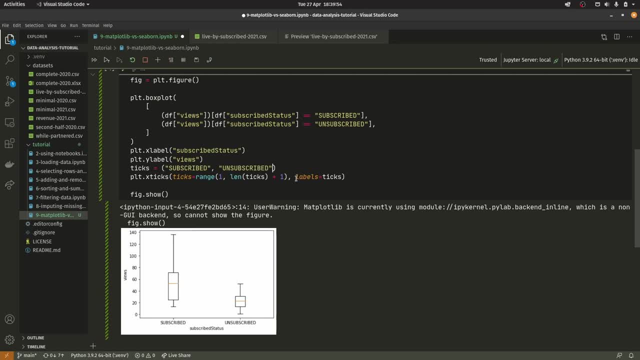 Yeah, you can. Okay, so that's the way around now. So, if I suppose order does matter, So you probably will actually want to use a tuple. But, as you can see, we have our graph here, If I make it a little bit bigger. 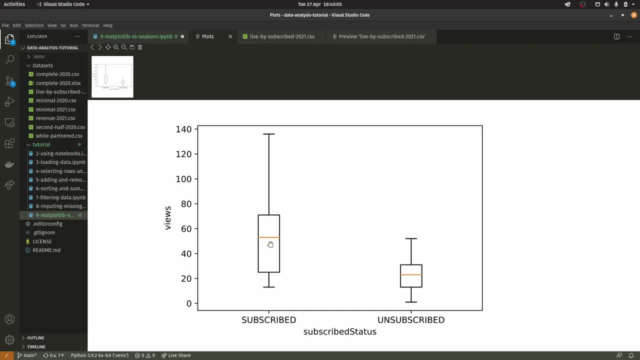 We have a graph here of, you know, my subscribed views on live streams and unsubscribed views on live streams. So, generally speaking, we're going to use a tuple. So we're going to use a tuple. So we're going to use a tuple. 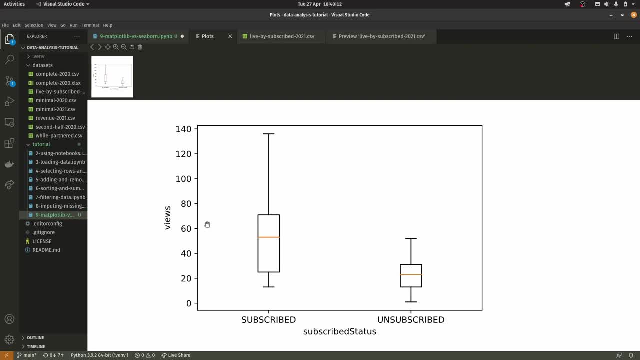 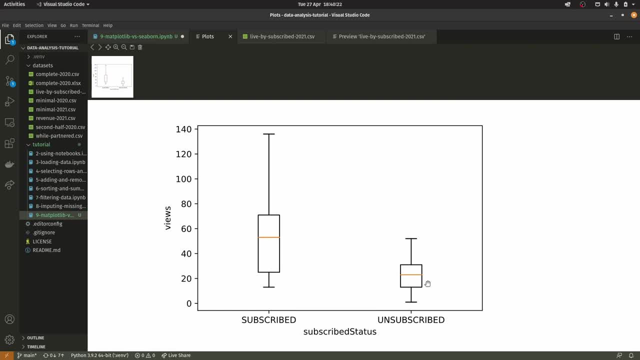 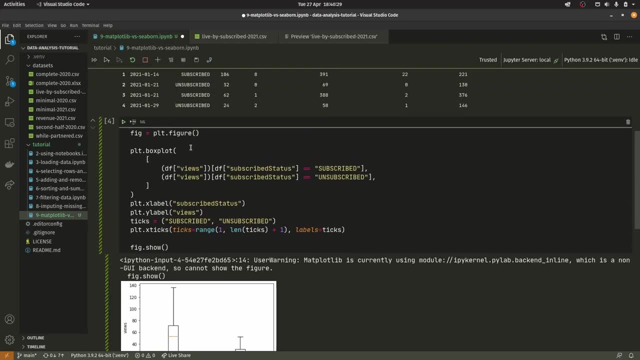 which I suppose it makes sense for streams. For videos, it makes sense to be the other way around, But for streams it makes sense to be this way around. So, as you can see, there's quite a lot going on here. So we create the figure. 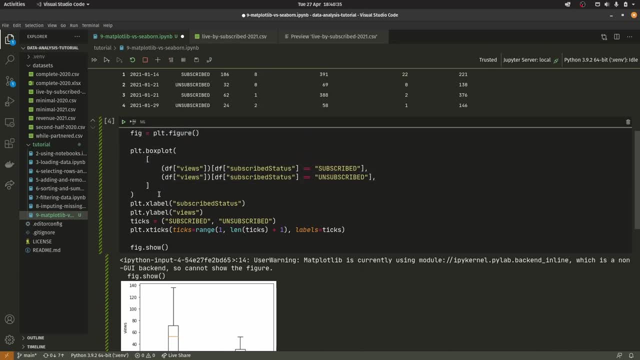 We actually tell Matplotlib what boxes we want to draw. Then we manually set the X label, Then we manually set the Y label, Then we have to create a list of ticks. This should really be tick labels, I suppose. Just make it a little bit clearer. 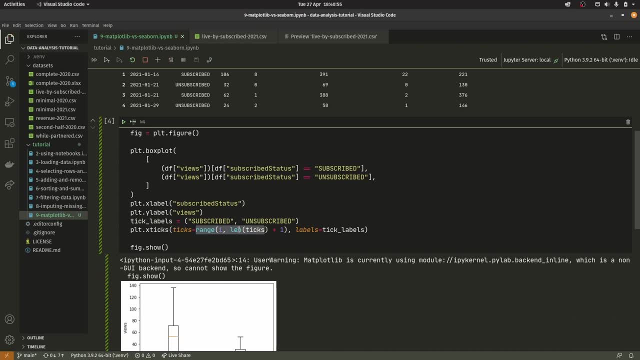 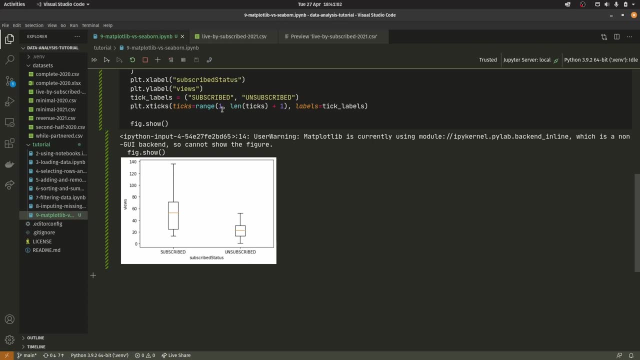 And then you actually have to apply these ticks. So you have the ticks and then you have to set. if you set it at zero- it's this line here- It will actually set it on the Y axis itself. So you need the one, and then obviously you need the length of ticks plus one. 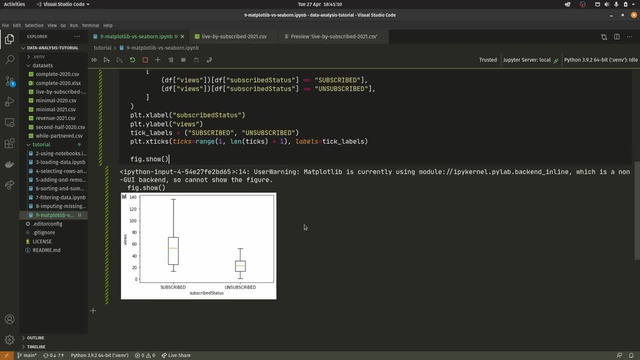 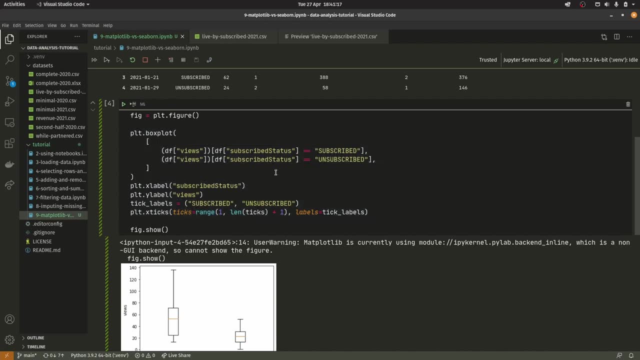 And you have to set labels to that And then you have to show the figure. So there's a lot that you have to do, But you can see how you have a lot of manual fine control over this, But a lot of the time you just want to get a graph out quickly. 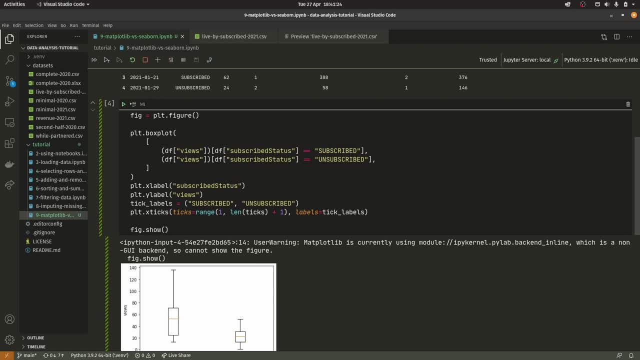 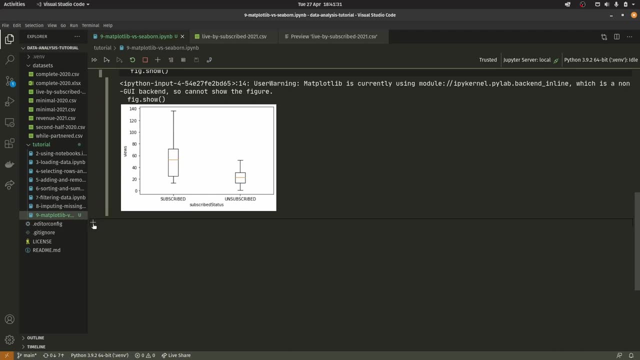 and you don't really mind too much about all the fine details. You kind of want something that can set these axes for you and all that. So this is where, as I said before, Seaborn comes in. So if you're doing Seaborn, it's a fig equals pltfigure. 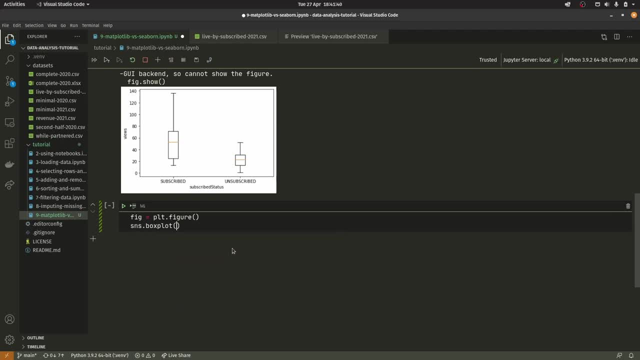 snsbox, Not box and plot. that's the wrong one. I'll get to box and plots later, But right now we're just doing a standard box plot. So data equals df. So we pass our data frame in. X equals subscribed status. 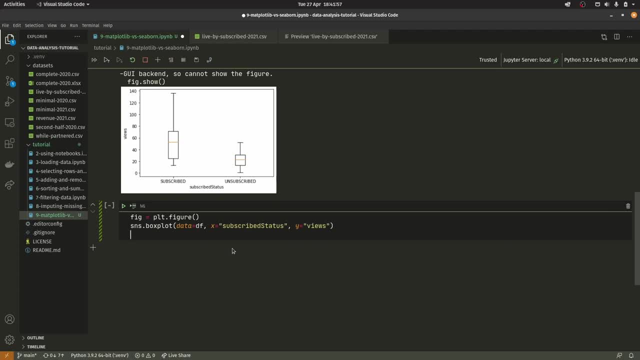 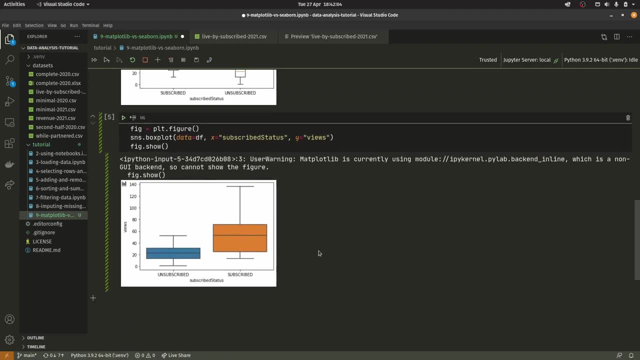 And Y equals views, And then figshow And voila, we have our graph. Now you can see that everything is backwards. I don't necessarily. I don't know why it does it Suppose if the order matters, I imagine there's probably a way to change it. 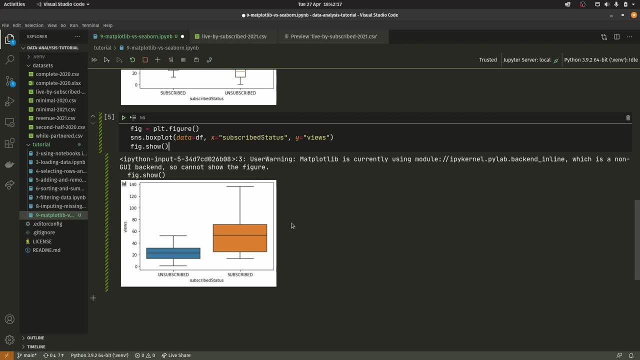 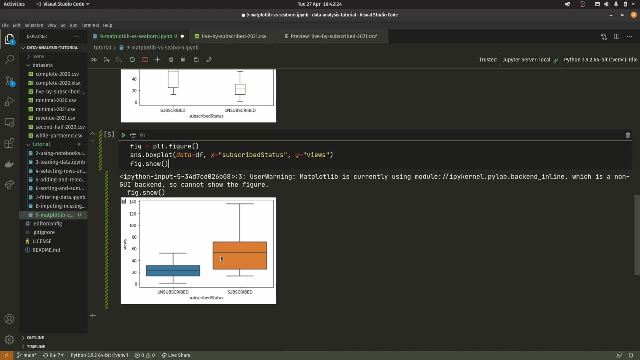 But in this particular example, the order doesn't matter at all. But, as you can see, there are a number of differences to talk about. So the first is the width of the graph- The widths are set differently- And the second is the color. 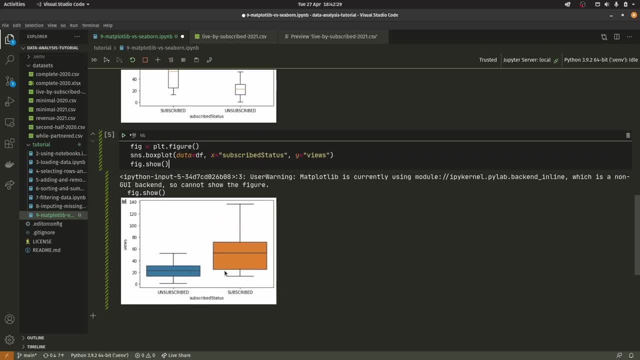 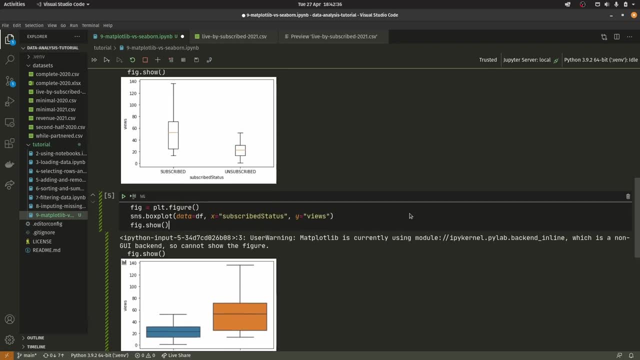 So the colors are set differently as well. All the colors are actually set to something in Seaborn And it gives you an actual, nicer looking graph than the one that Matplotlib gives you out of the bat. It also gives you the X ticks automatically. 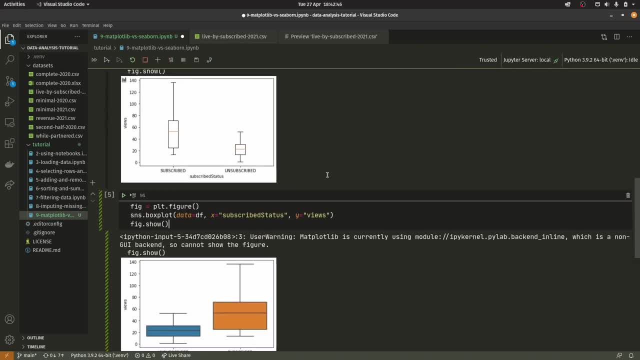 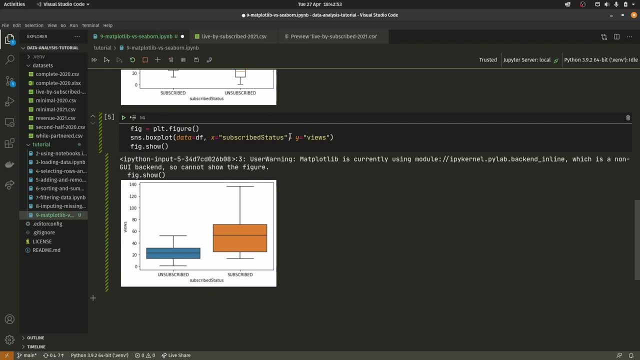 And it also gives you the labels automatically as well. So you can see, all this stuff is exactly the same as it is in the Matplotlib one as well. The only difference is the way that this actually performs these operations. So essentially, we're passing in the data frame. 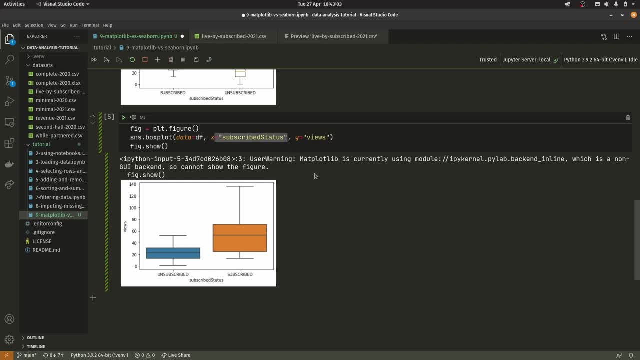 So we're saying this is the data we want to use. The X axis is the subscribed status. So because there are two different values that are possible In this column, it gives us two hotspots. So there's unsubscribed and subscribed. 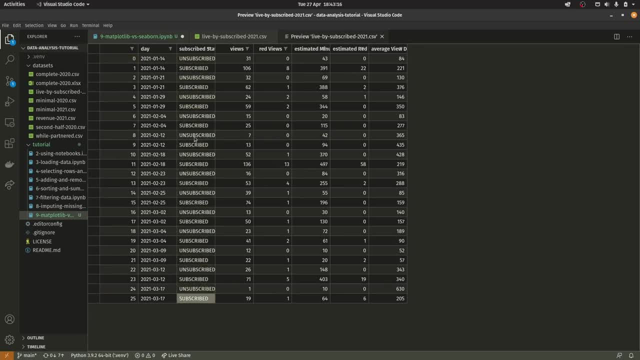 Look, as you can see, these are the only two values you can get. If there are more values, then you'd actually have them all, And if you're doing device type, for example, there are a lot more device types And you could just pass in X equals device type here. 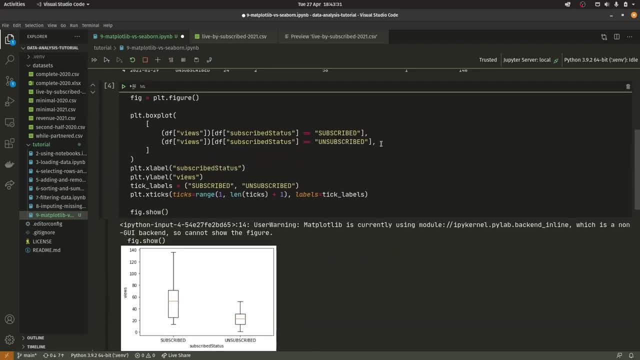 And it would automatically create a new one for you. With this, I mean, we only had to do two, But if there were more than two, then you would have to do all of them manually, Unless there is a better way of doing it. 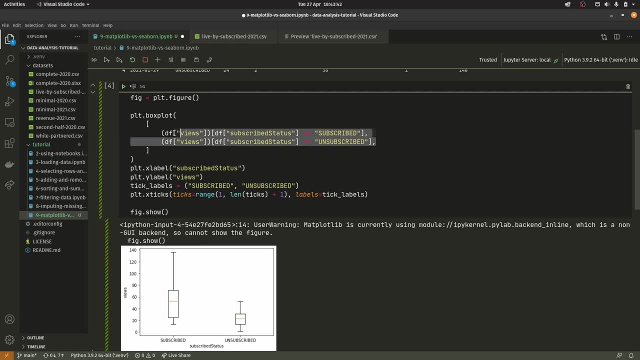 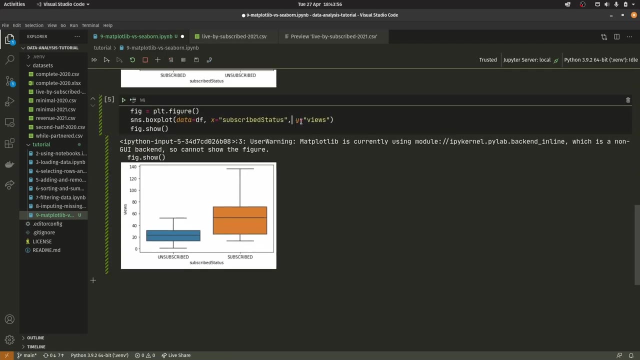 which I don't know. There probably is some sort of way to get this to split like that dynamically. If someone does know, then let me know, But I don't know it. And then, of course, you have the Y equals views, which is the same. 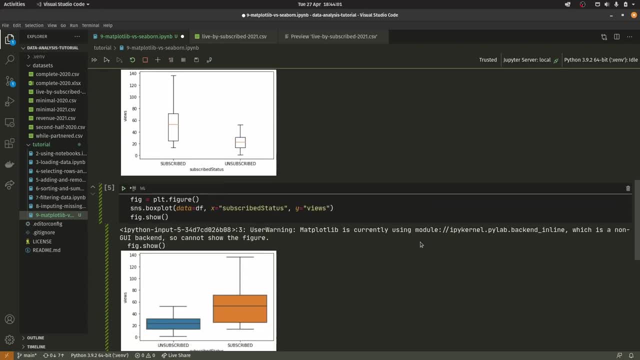 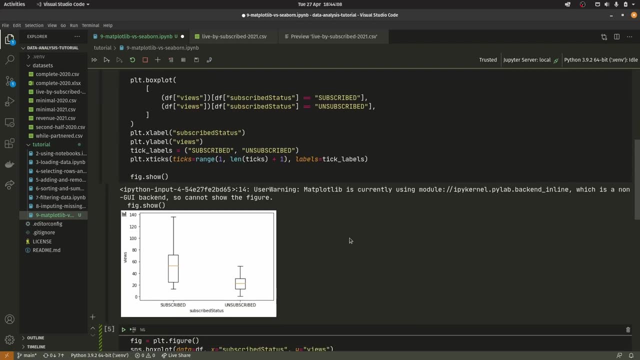 So, as you can see, these are the differences. We're going to be using Seaborn throughout the rest of the series, because it is just a lot quicker and a lot easier to use than just straight up Matplotlib. Of course, straight up Matplotlib does have its uses as well. 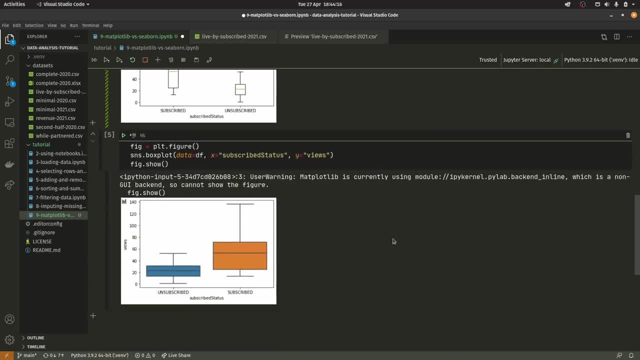 but not really in this series. We just want the graphs to look nice. We want the graphs to just make themselves. It's all automatic with Seaborn, It's all done for you, And that's what I like about it so much. 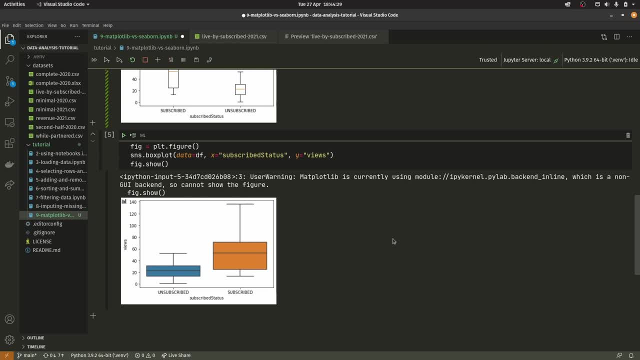 But yeah, that's all I really wanted to talk about with comparing these two different libraries. If you have any questions, then feel free to leave them in the comments below, Or you can join the Discord using the link in the description. But yeah, with that, I'd like to thank my patrons for being as amazing as they are. 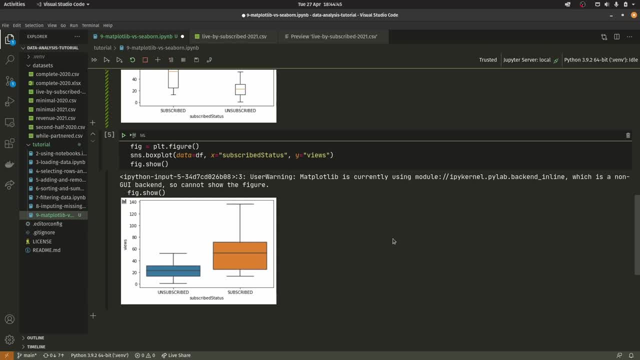 And I'll see you next time. Bye, I'll see you next time when we actually start doing some actual graphs and I explain kind of what they do. So we're going to be doing line graphs, scatter graphs, rug graphs and ECDF graphs in the next video. 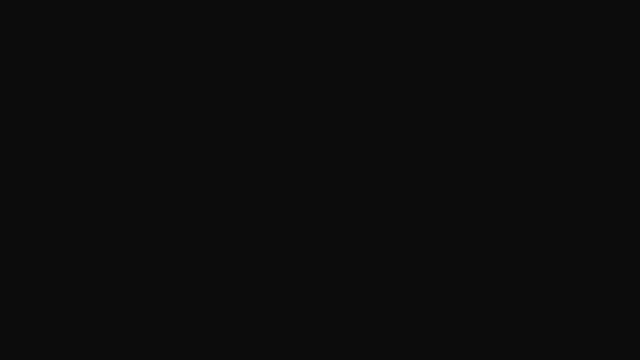 So I'll see you for that. I'll see you in the next video.